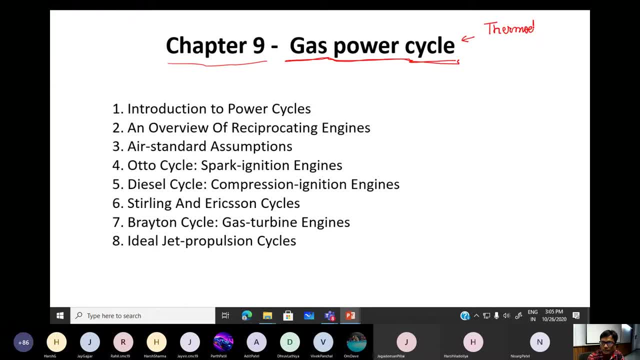 thermodynamic cycle. So this is one type of thermodynamic cycle We are going to look in this particular chapter is gas power cycle. There is another cycle, power cycle, which is known as vapor power cycle and which we are going to seek in the 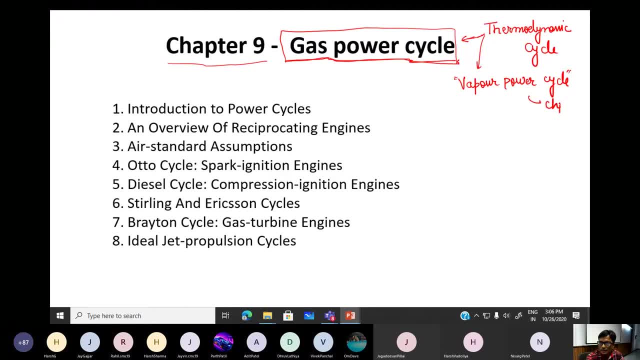 chapter 10, in the next chapter, Namely this gas power cycle is a type of thermodynamic cycle, which is a thermodynamic cycle which whose working fluid, whose working fluid is single-phase gas, single gaseous phase, Okay, Whereas this vapor power cycle contains two-phase or multi-phase. 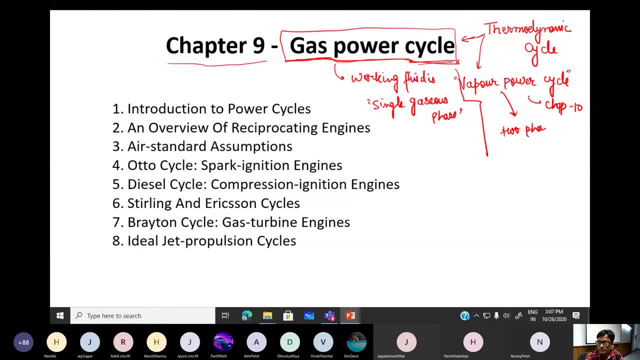 So in essentially, these two phases are not parallely present. Essentially, in one part of the cycle your phase may be liquid and in the next phase- it could be sorry, in the next process it may be liquid. Okay, So temporarily engaged within этому. 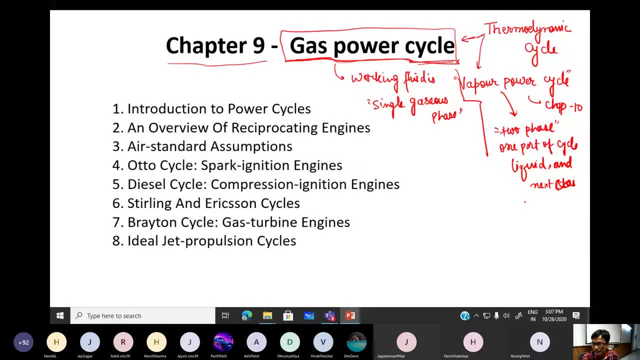 cycle cycle, not cycle next part of the cycle. part of the cycle it may be gas. So in this particular chapter we are going to focus only on the power cycles or the thermodynamic cycle whose working fluid is a single gaseous phase, that is mostly air, will take up in this particular 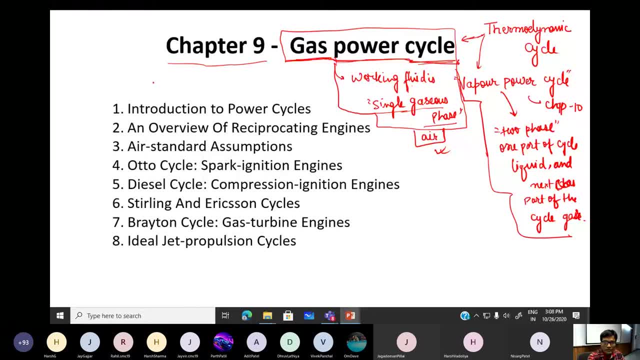 chapter. So the overview of this chapter is: we are going to start with the introduction of power cycles. what are the various types? gas power cycles and vapor power cycles, and different classification. there are open and closed thermodynamic cycles, there are internal and external, So internal combustion engines, and so Next we are going to take up the overview of an 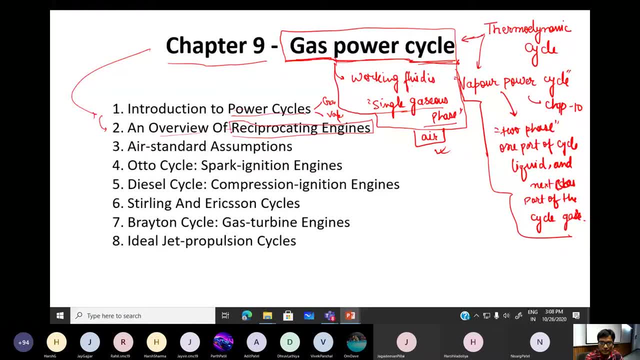 reciprocating engine and which is which would be the main focus of this particular chapter. Essentially this, reciprocating engines are more widely used in your automobiles, So we are going to take up the assumptions based on which your these cycles work and which. 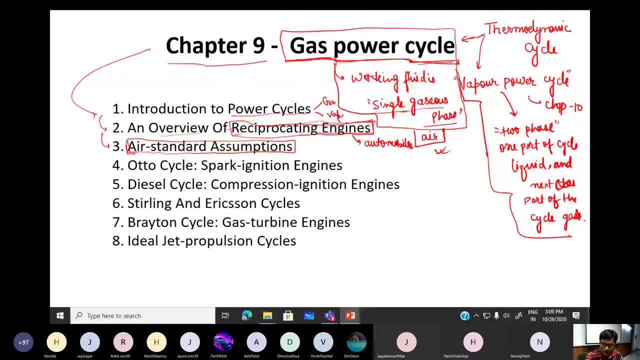 is also called air standard, assumptions that we are going to take up in order to analyze the thermodynamic cycles that are involved in reciprocating engines or gas power cycles. There are two types of thermodynamic cycles: One is the gas power cycles and the other. is the thermal power cycles. The first is the thermal power cycles and the second is the gas power cycles. The second is the thermal power cycles. The third is the thermal power cycles. This is the thermal power cycles and the fourth is the thermal power cycles. 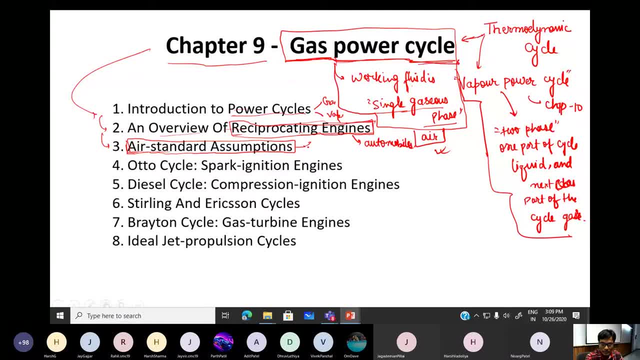 So these are the two types of gas power cycles that are widely used. we are going to cover that Auto cycle and diesel cycle. Auto cycle is also called spark ignition engine. I mean this is the ideal cycle which we are going to take and based on the application is application. 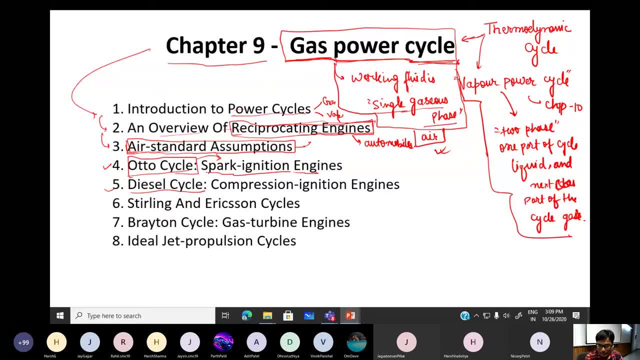 wise it is. it is used in the engine which is called spark ignition engine and which is which works on ideal auto cycle, And we will look into details about the engine in the next lecture, how this, these engines work, the second type, second type of cycle that we are going to read. 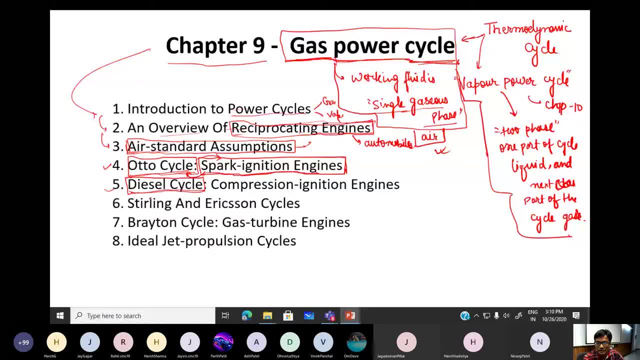 in this particular class is the diesel cycle, the idle diesel cycle and the application wise compression ignition engines. that works essentially based on these diesel cycles. there there's in some in some process wise. there they are in some sense deeper and in the cycle manner. so that is why we have two cycles and we look in more into the details when we look further. 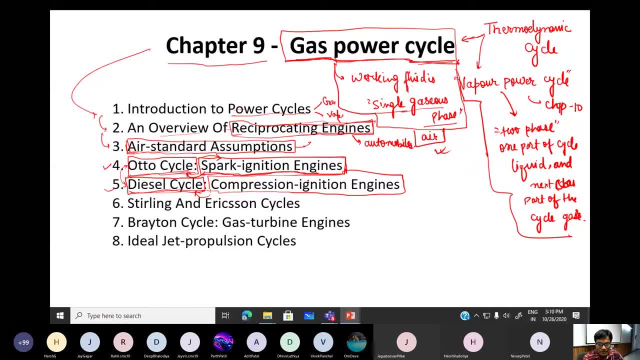 there. there are few other modified thermodynamic cycles through which some engines work, namely Ericsson and sterling cycles will also look that, not in details, but yes, we will get into touch with these cycles. second last, we are going to take up the Brayton cycle which is of often used in gas turbine engines. you are: 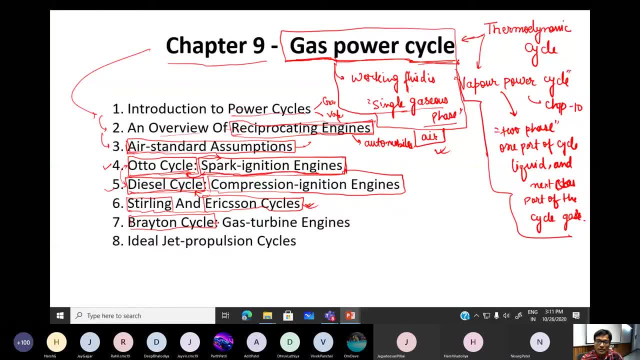 going to take up some mechanical advantages, mechanical work from turbine, those, those are based on Brayton cycles and, lastly, we will take up the idle jet propulsion cycles, which is close, which is very much close towards Brayton cycle. but the only difference is here you have a nozzle through which the gas is being expanded through, 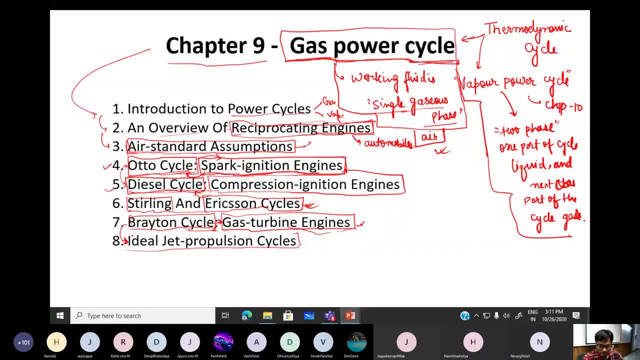 which you get thrust, and this type of thermodynamic jet propulsion cycles are used in aircrafts, aircraft engines, the ramjet huh. there are different types of jet propulsion engines: ramjet, scramjet, foreign. okay, yes, so this would be our overview of this particular gas power cycle. 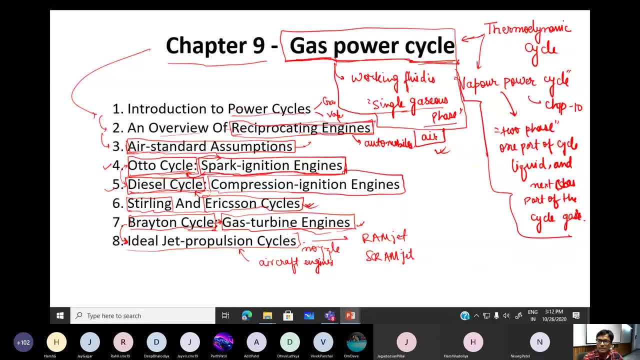 so we are not going to take up a vapor power cycle in this particular chapter, since it it has the philosophy of the different working fluid, which is having two phase. ok, So we will stick on gas power cycle in this particular chapter, since your working fluid is single gaseous phase. that. 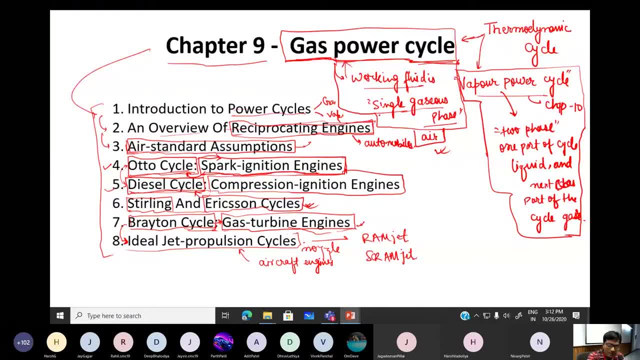 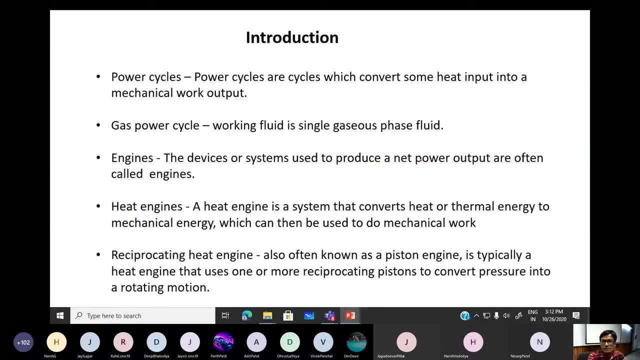 is air. ok, To start with the introduction, so we already know that. what are thermodynamic cycles? So what is cycle before I mean? what do you mean by cycle When a process, when a process or when a thermodynamic process starts from one? 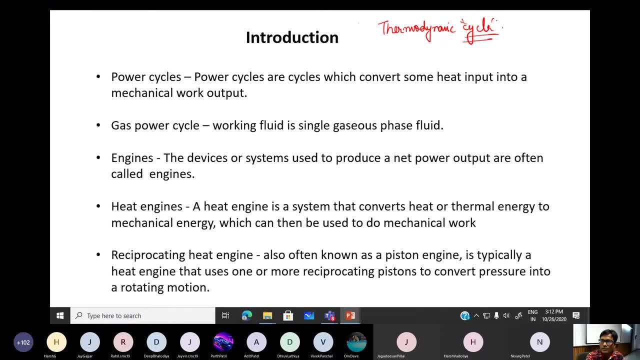 initial point and it comes back after doing some other process and comes back to the same position. So we call this kind of on some- let us suppose P V plot or T V plot, ok, If you start from one state and you come again and arrive at same state. finally, you call these kind of. 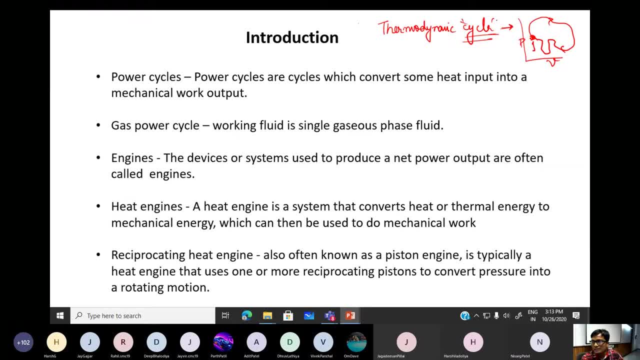 process is cycle ok, And these cycles are advantageous in a way that P can get the work out of it- advantageous work out of it. ok, And the power cycles. the power cycles are cycles which convert some heat input into mechanical work output, which 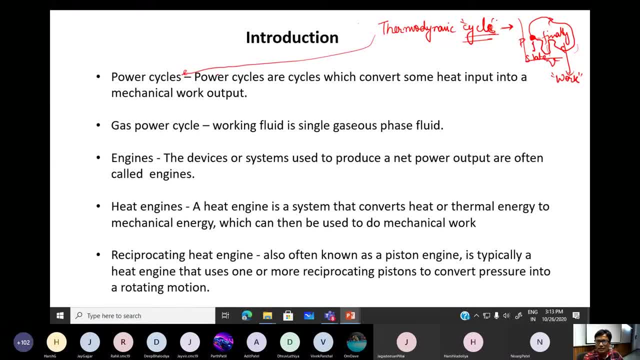 is similar what I told here. ok, And yes, the gas power cycle is defined as the power cycle which. So we are going to start this with a single part of the liquid in which the working fluid is single gaseous phase fluid. example: air. In this chapter we will take up the air as 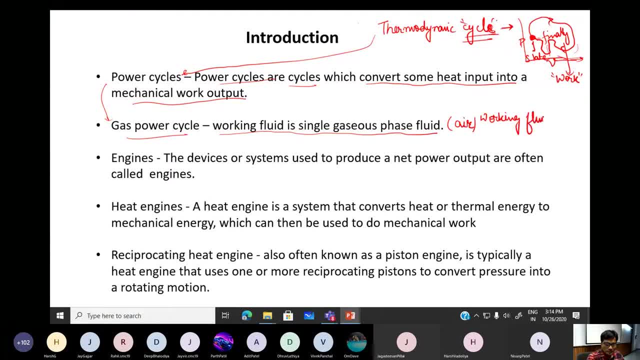 my working fluid for all my cycles. We also should know about the definition of engines, So there are few key words that I am going to oftenly use in this particular chapter: engines, heat engines or reciprocating heat engines. So I am going to now talk about the energy generation, And this is the main. 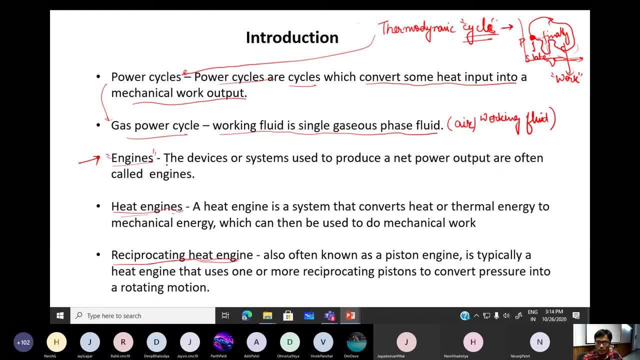 So engines are. the devices or system used to produce net power output are often called engines. Any device that produces advantageous work or advantageous net power output is called engine and does not matter it works on heat or chemical reactions or some other means of energy. 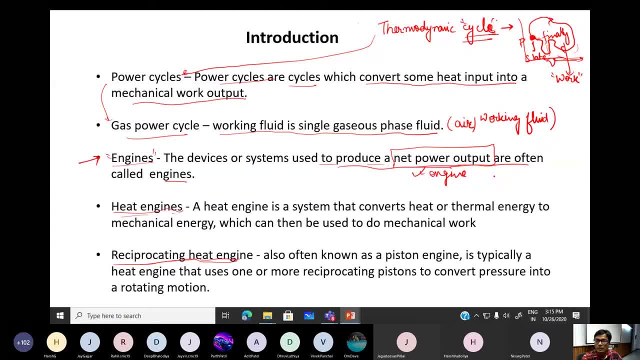 If it produces some advantageous net power output. we call this as engines, whereas the heat engines are defined as the heat engine is a system that converts heat or thermal energy to mechanical energy, precisely So this is a type of engine which converts heat or thermal energy to mechanical energy. 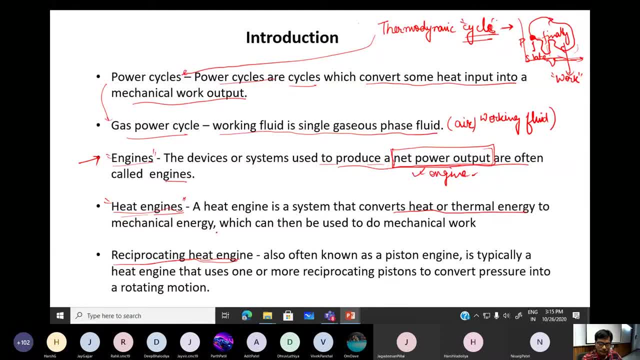 and which can then be used to do mechanical work. Are there any other questions? Type of heat engine is we are going to often take up in this whole chapter- is reciprocating heat engine, also often known as piston engine, is typically a heat engine that uses one or 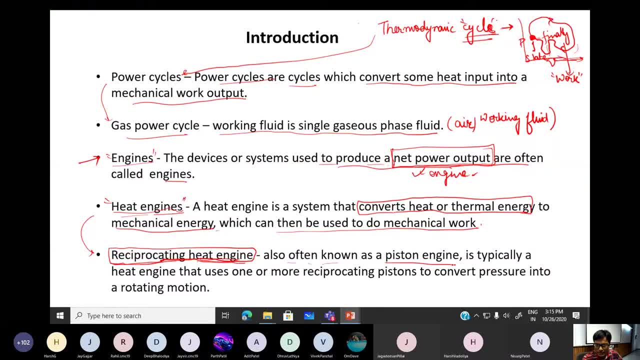 more reciprocating piston to convert pressure into a rotatory motion And we will see in details, in very much details, about this reciprocating heat engine. But we are going to study further in detail. We should also know the start. where does this heat engines and this combustion internal? 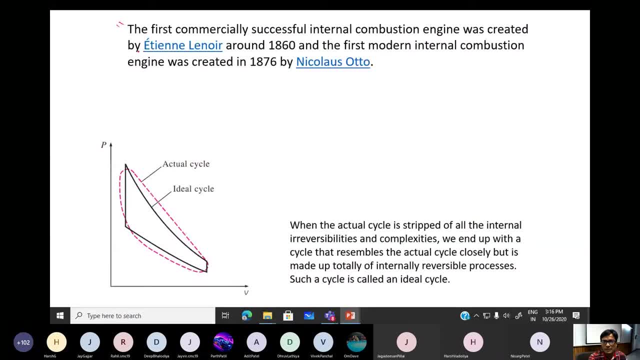 combustion engines or reciprocating engines first starts. The first commercial successful internal combustion engines was created by Etienne Lenoir around 1860.. The first modern internal combustion engine was created in 1876 by Nicolas Otto, after which our Otto cycle, the cycle, is named after this scientist. 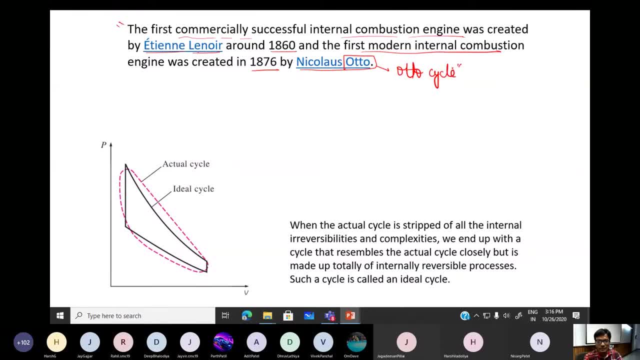 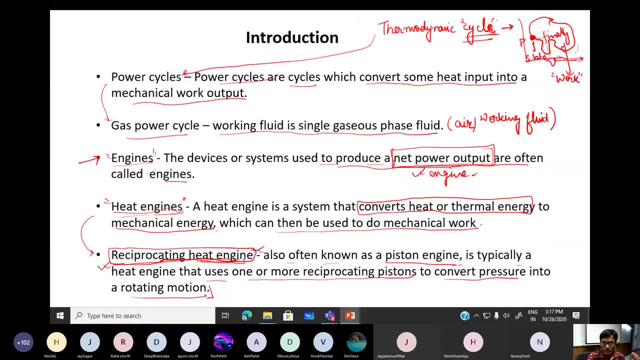 So internal combustion engines- okay, so I missed one thing here. This reciprocating heating or the heat engines may be classified as two types of engines. One is internal combustion engine or another is external combustion engine. So internal combustion engines are the engines where the working fluid is being heated internally. 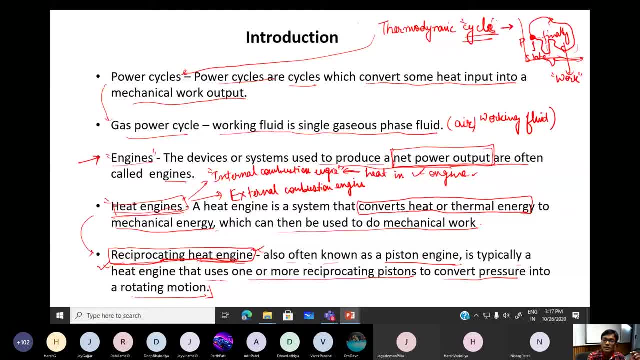 Okay. heat is given to the system when your control volume is chosen and your heat is being produced inside here itself, I mean internally, within the control volume- whereas the external combustion engines, such as I mean this- the example of this internal combustion is your autumn oil engine- whereas this external combustion, in this heat, is being supplied. 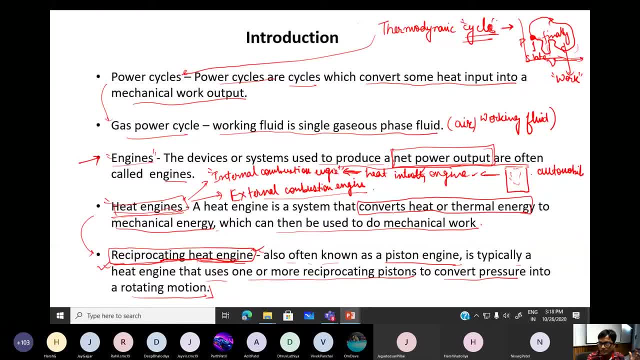 to the system externally. So from some working fluid is being heated somewhere and it is being brought into the system. later Heat is being inputted externally and then it is being brought to the system. So one such type of external combustion engine- you can think of a steam power plant. 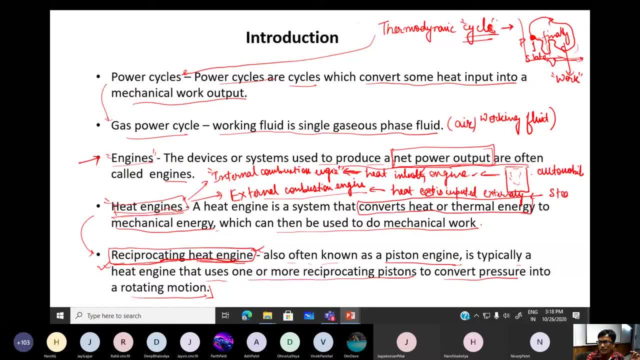 Okay, So in boiler, your steam is being generated by heating up the water externally, okay, and then it is flown through turbines to get the power output. Okay, So, yes, So. So the first internal combustion was created way long back, and still we are in a philosophy. 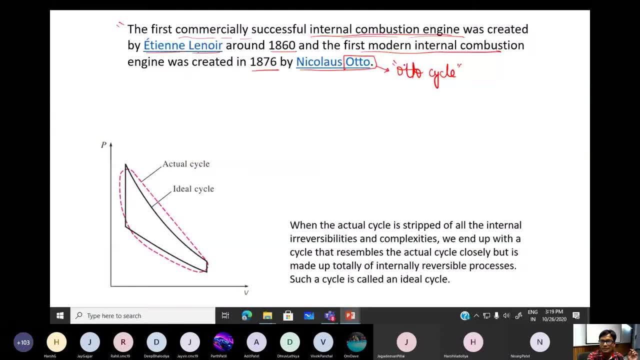 to make things more efficient. that is what our I mean. modern, I mean, if you want to work with it, you can make it work by using a steam engine. Okay, So that is, you know, a steam engine, and if you have a steam engine, you can make it. 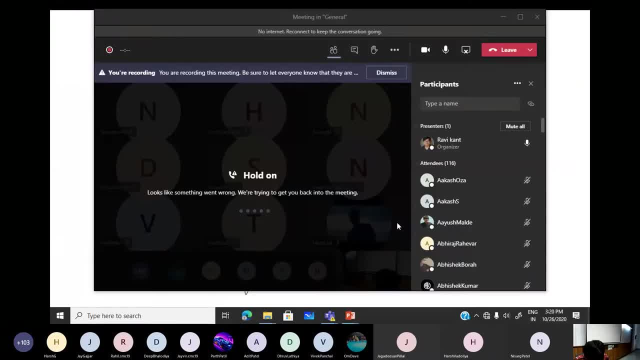 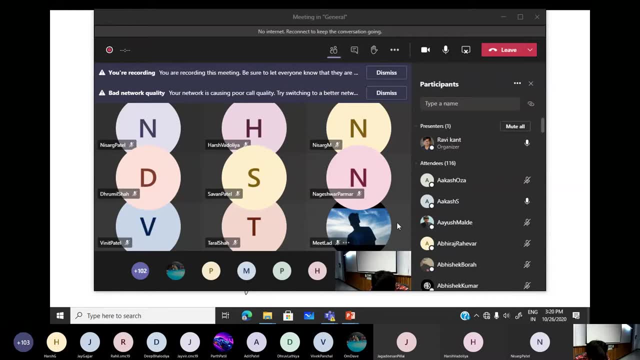 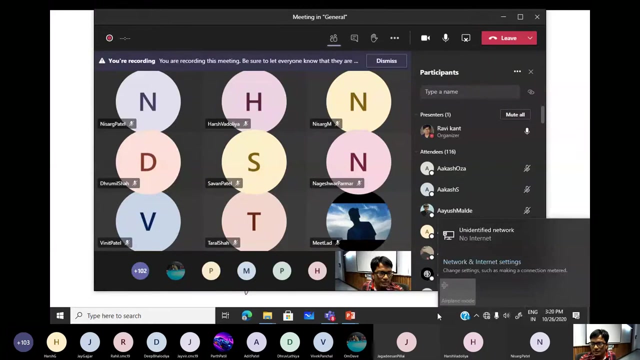 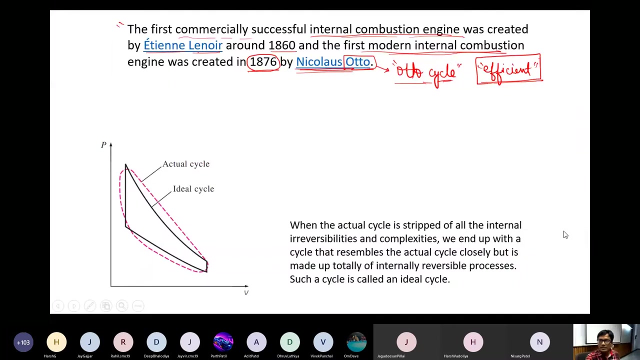 work through a steam engine. Okay, Okay, Yeah, Yeah, okay, uh, am i audible? like there was some internet problem here from this side? yes, sir, oh, it's audible now. okay, so i was, i was, i was telling that, uh, i mean the the modern day, uh, study. 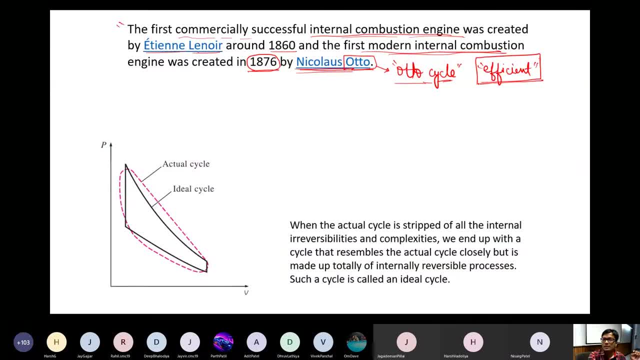 on internal combustion engines are basically how to make it more efficient, and so, because the the basic cycles were already being given 1800, we are in a phase to make it more efficient. that's it what we are currently doing, actually. okay, uh, next thing i want to talk about is 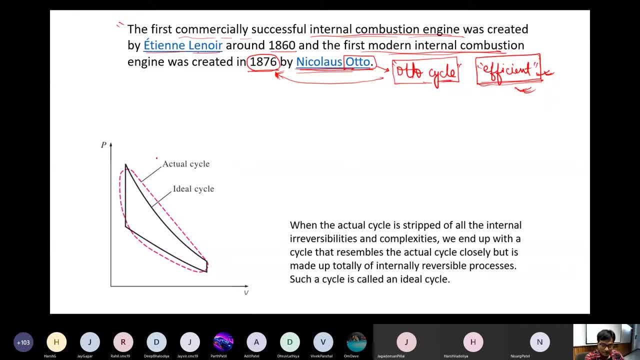 the actual cycles that in, in reality, what these inner internal combustion engines are in this red dotted process you can see from. it may be going from some, some state, one, two, two, by some two, three, four and something, but we are going to analyze this particular actual cycle. 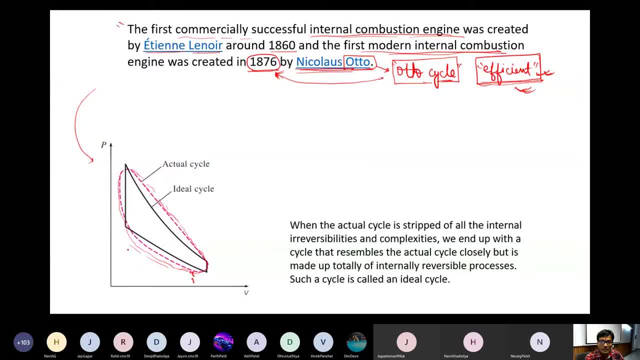 through this idle cycles okay, the reason being: it is easy to analyze without giving up on the errors, giving on accuracy, okay. so even if i am idealizing it through idle cycles, such as auto or diesel cycles or breton cycles, even though i'm idealizing it, nevertheless i'm not giving up the accuracy because when the actual 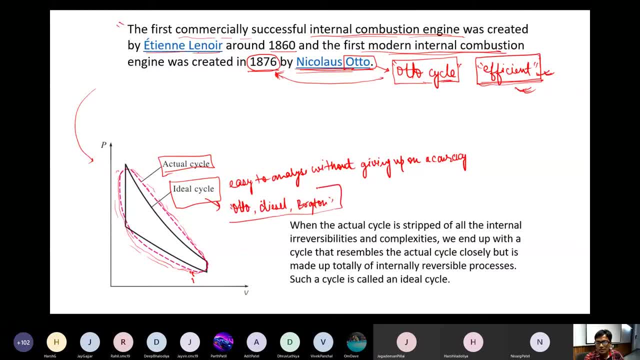 cycle is stripped off all the internal irreversibilities and complexity, we end up with a cycle that resembles the actual cycle closely, but it is made up of total internal reversible processes, processes. So we are not giving up on the accuracy. such cycle is called ideal cycles. 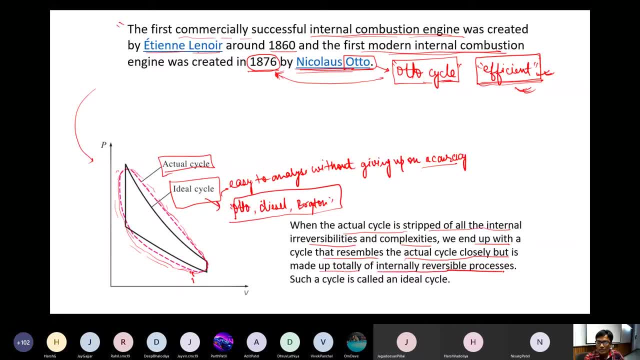 and we are going to analyze thermodynamic, all the formulas and all the essential analysis. we are going to talk in reference of these ideal cycles, not the actual cycles. we are not going to analyze these actual cycles in reality. ok, In reality we are going to talk. 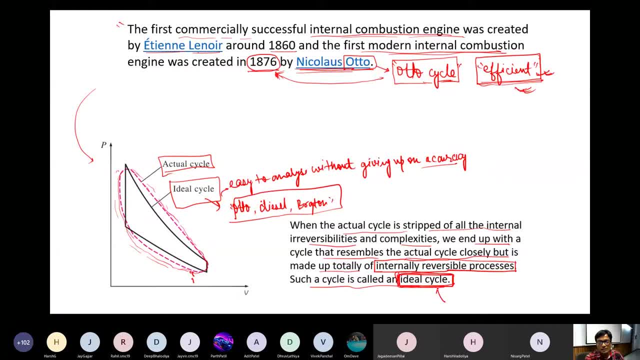 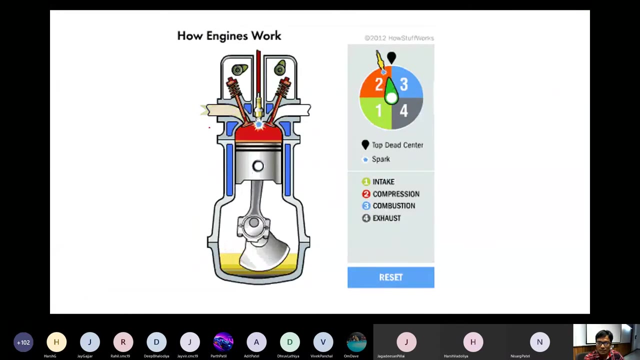 about the ideal cycles which are close towards these actual cycles. A typical engine schematic or animation shown over here: this is internal combustion engine. So you can see, let us suppose it starts from 1. ok, So 1 is your intake, So intake is getting. 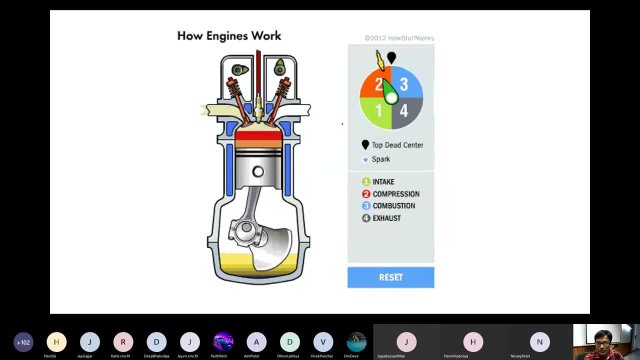 getting fuel, air, fuel mixture, from this left side and valve is being open from here to here, from process 1 is and after that process that happens is called compression. Ok, So in in compression we will talk about in details of what what is happening, but just 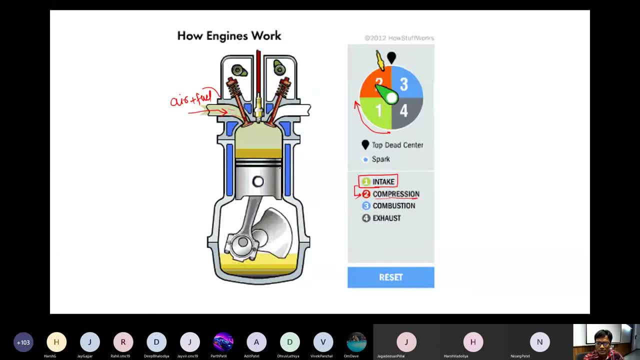 to give you an overview of how these engines work, just to guys you, to motivate you, this is the animation of it: first the intake is happening, then the compression is happening by the means of this piston cylinder arrangement and then, due to this, this spark plug, the spark. 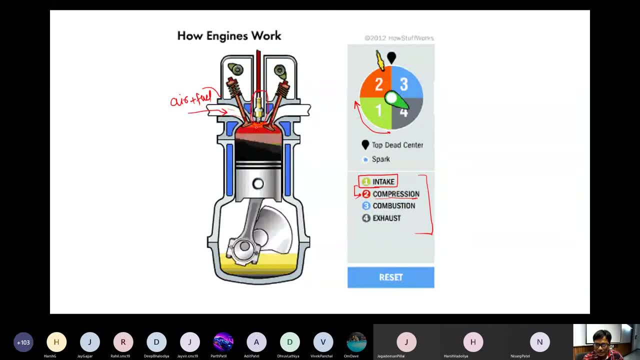 happens and Ok. Ok, So this is the piston cylinder arrangement and this allows this air fuel mixtures to burn or to combust and it increases the pressure and the temperature and in turn it, due to this large pressure, you can actually push this piston to and fro, and this piston is. 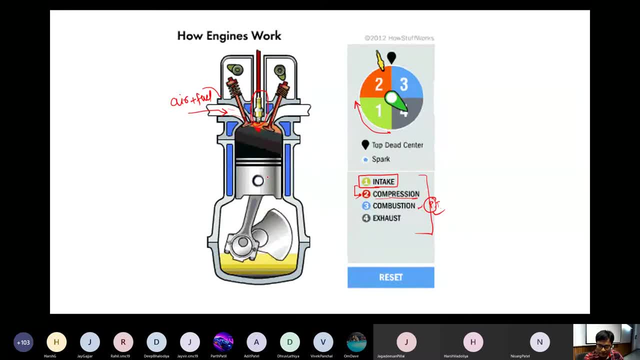 being connected through the connecting rod and it is finally connected to the crank shaft. and in your kinematics of machine You can- I mean you might be knowing that because, due to the reciprocating motion piston, the crack crank shaft revolves and this revolution is being connected to the gear, gear boxes. 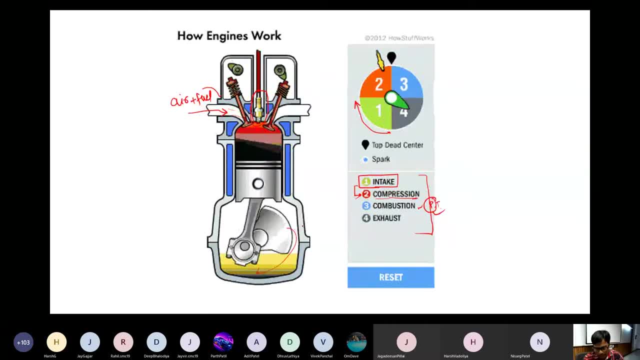 and through. I mean with particular speed or whatever the desire desirable torque you want. you can provide this torque or this rpm to your wheels. Ok, And finally the left over gases. the are being exhausted at the later stage. So this is typically for process. it undergoes a typical internal combustion engine. 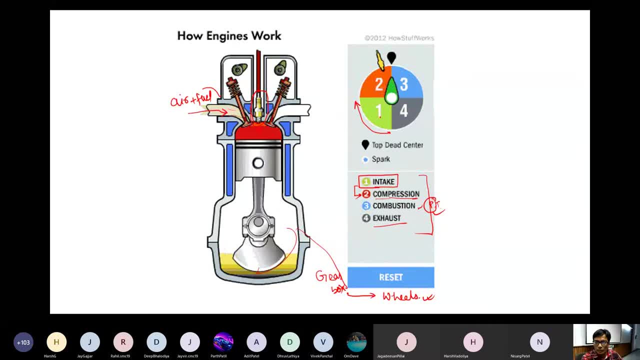 So essentially it is IC engine or more precisely spark, SI, spark ignition, internal combustion engine. Ok, And this is also 4 stroke. We will see. what are these key words? 4 stroke, 1 cylinder or 4 cylinder, we will see in more. 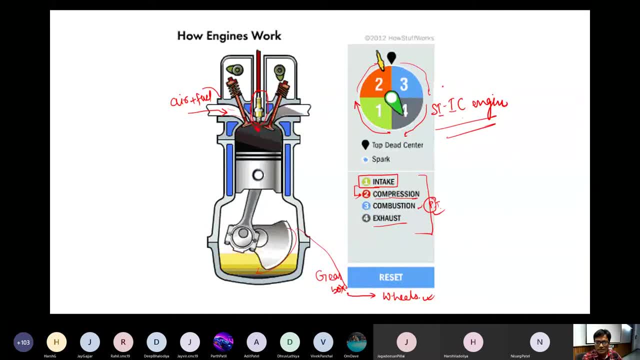 details. So this is particularly: you have 1 cylinder and if you have parallely 4 cylinders doing the same thing in cycle, I mean there are 4 pistons in it and parallely it is moving and it is providing the torque to the crank shaft, parallely it will give you, I mean it will be. 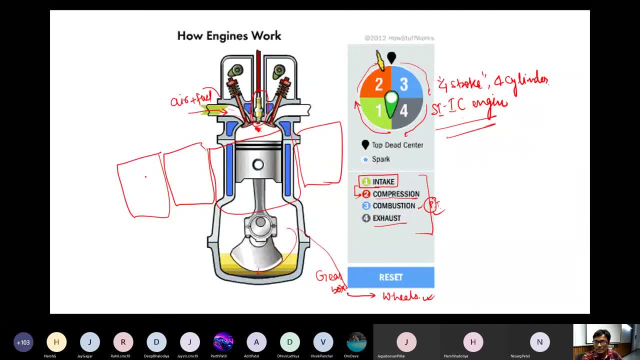 told that it is 4 cylinder And 4 stroke is nothing. but in 1 cycle, in 1 complete cycle, it crosses 4 to end, flows from top dead center to bottom dead center and this is why it is called 4 stroke. 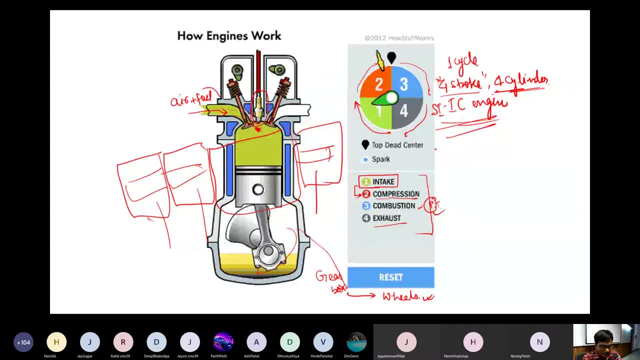 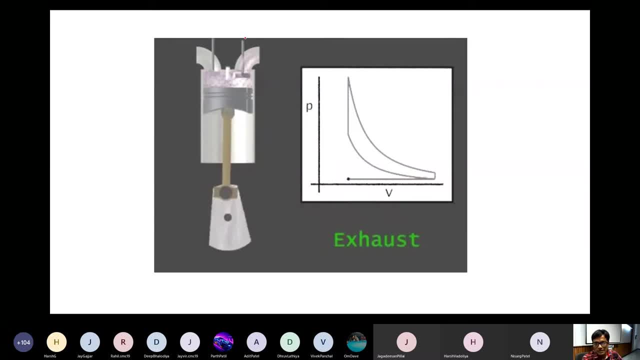 So we will talk in details in the subsequent slides. this is more realistic. I mean, this is an animation. So 1 stroke plus 1 cylinder and 1 cylinder goes to 2 cylinders. so it goes 2 cylinders and 1 cylinder goes to 4 cylinders. 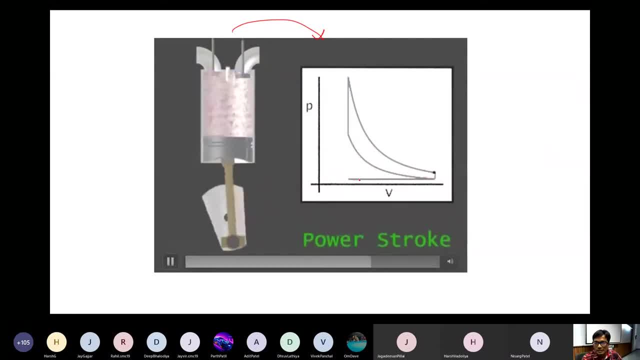 So for a specific type of engine, the crank shaft or the engine itself can be set to the max diameter 5.. So at least it is possible to do this. we will see the same thing for a crank shaft or a canister, Ok. 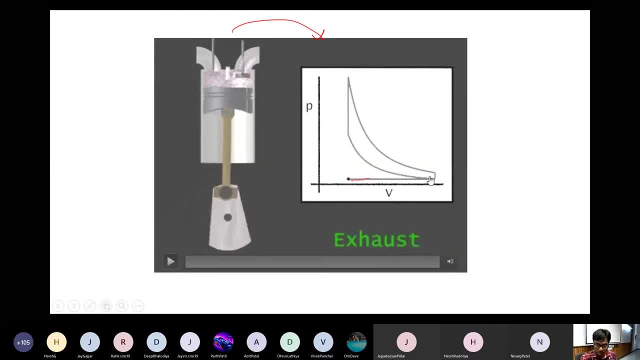 So let us okay, adiabatically, compression is happening at constant- sorry, constant- volume, the heat is being added and then the power stroke is this and then exhaust. so this is a typical auto cycle that we will look and diesel cycle is constant volume process, heat addition process. 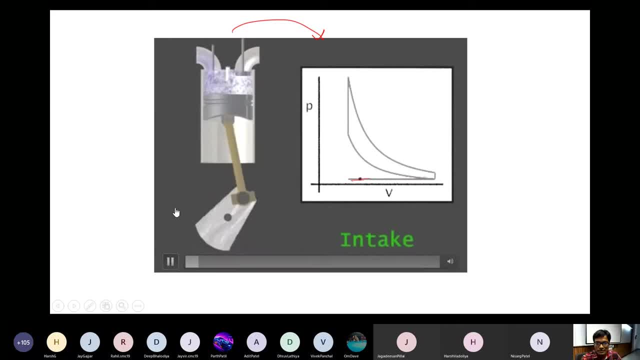 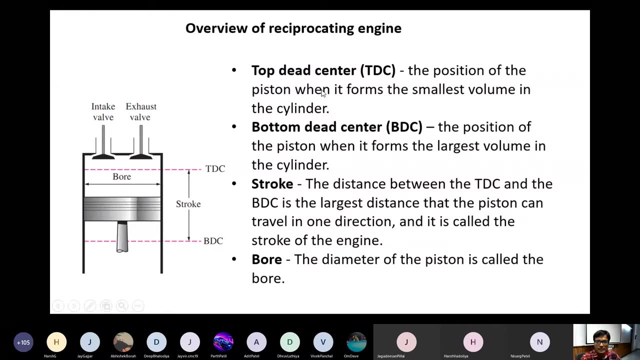 is there. we will look into- but this is just to motivate you guys- what is happening inside this particulars piston cylinder arrangement or the IC engine. ok, So, as an overview of reciprocating engine, we are going to look up few nomenclatures, which is essential part of understanding the IC engine. 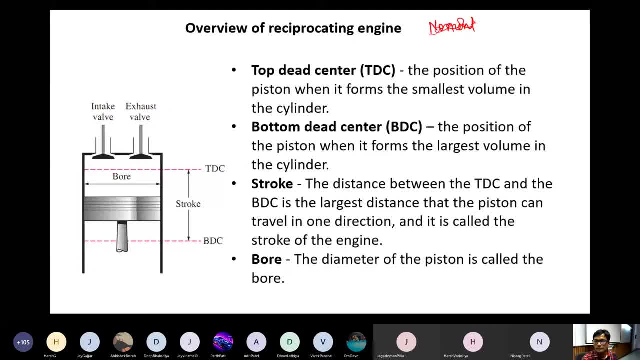 So some few nomenclatures such as we will be frequently encountering, such as stop dead center, TDC- you guys might have heard about this. This is nothing but the position of the piston when it forms the smallest volume in the cylinder. So this piston- initially it was here. 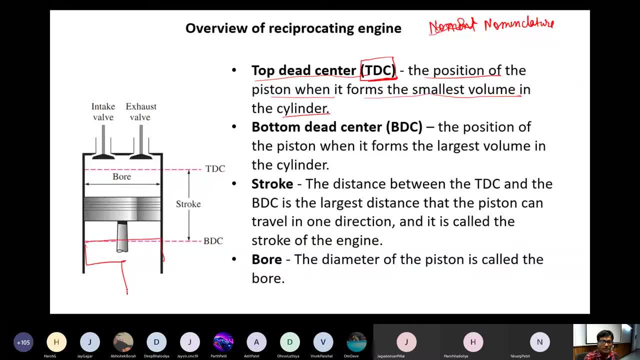 And because of the air pressure, it was here and it may go to and fro and the maximum up position it can go till here And this position is called top dead center, where the volume of the air is smallest volume that it captures this air, air fuel mixture is coming from here and exhaust is here and 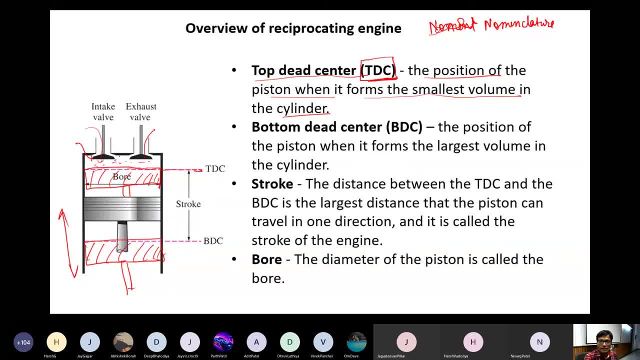 this place, this volume you can think of as a smallest volume that it can have at any moment of time, and this is called, and this position is called actually, TDC. The bottom dead center is the position of the piston when it forms the largest volume in the cylinder, when even it, when it is far away from this. 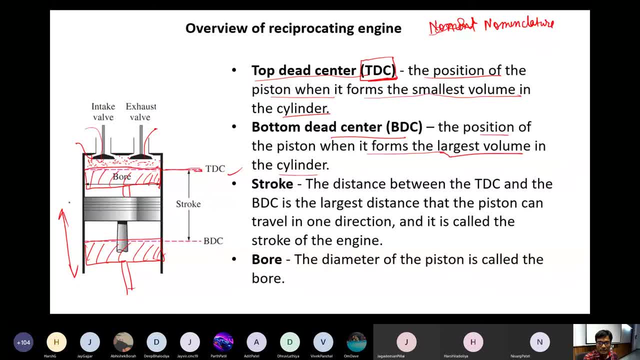 So this is the position of the piston when it forms the largest volume in the cylinder, when even it, when it is far away from this Note. the reason behind this is from machine model, usually On the same set of Mary 12. this has the 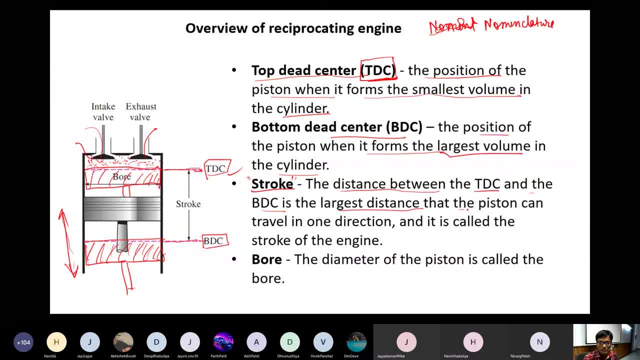 numberى number you have to. somethin is called stroke and it is often, uh, denoted by l subscript capital. l next thing is also often used is the bore. bore is is the diameter of the piston is called the bore. so so essentially this: your piston is, is your actually a cylinder? 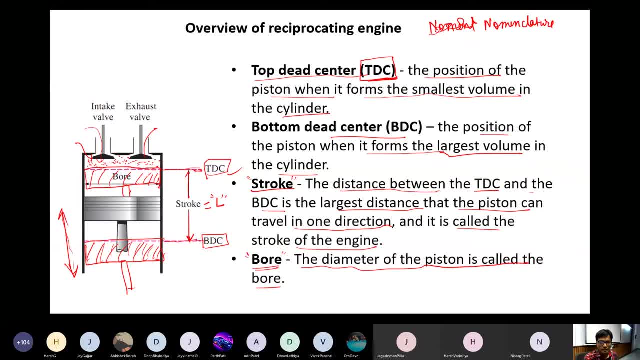 so this is this. this volume is basically a cylinder and your piston is: look something like this: this is your connecting rod and, yes, this is your. there are some piston rings will be there so that there should not be any leakage of the gases or, you know, the oil should not leak into. 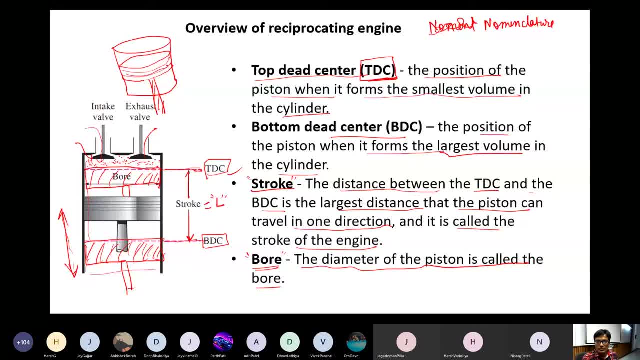 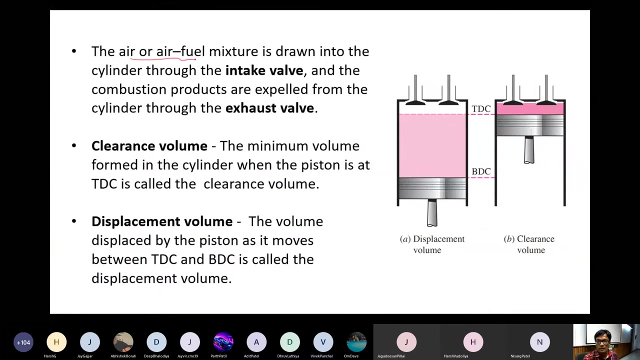 the combustion chamber. okay, so this diameter, this diameter d is called the bore, the air or the air fill mixture is drawn in the cylinder through the intake valve. so this valve is called intake valve, intake valve and this another valve is called exhaust valve. so these valves open and closes synchronously and then closes. 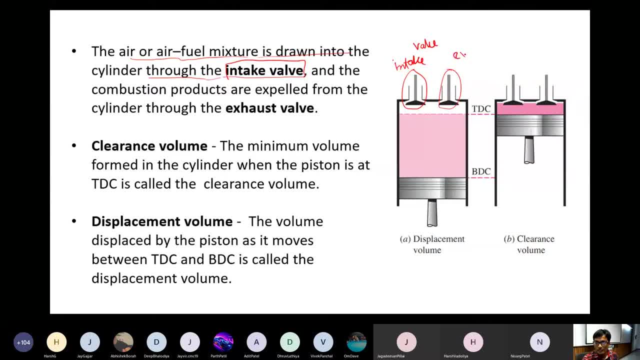 in sync. okay, in proper syncing. okay, without syncing uh, the gases will escape at intermediate time, so that will not be desirable for uh engine to work, so it should be in sync. and the combustion products are expelled from the engine to work, so it should be in sync. 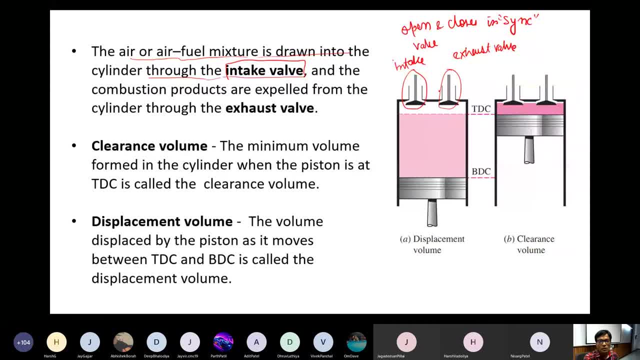 and the combustion products are expelled from the engine to work, so it should be in sync. and the combustion products are expelled from the engine to work, so it should be in sync. so there is something called clearance volume, the minimum volume formed in cylinder when the piston is at. 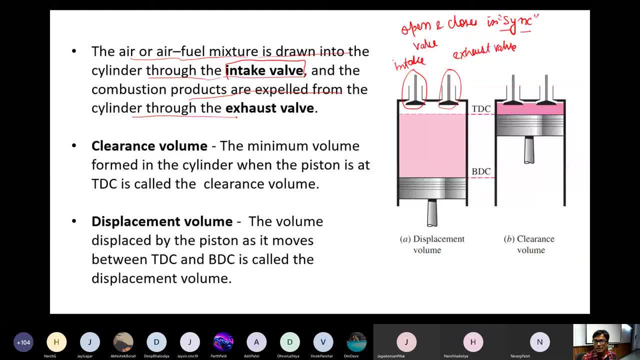 tdc is called clearance volume. so when your piston is at the top, most position, the volume that it contains, the gases, residual gases contains all the time, is called the clearance volume. this volume, let's see essentially this volume, these volumes, I mean upper volume- it's called clearance. 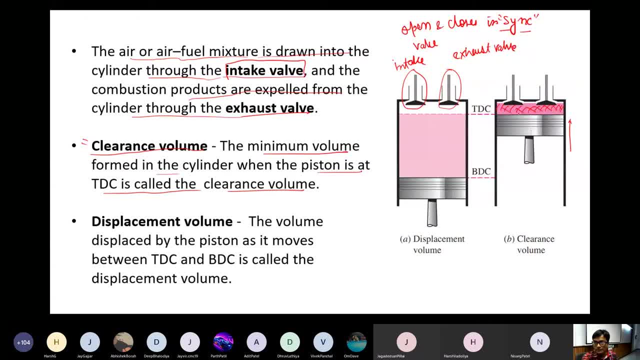 volume, sorry, clearance volume and displacement volume. there is something called displacement volume as well. the volume displaced by piston as it moves between TDC and VDC is called displacement volume. So this the left over, I mean from TDC to VDC, this L length times. 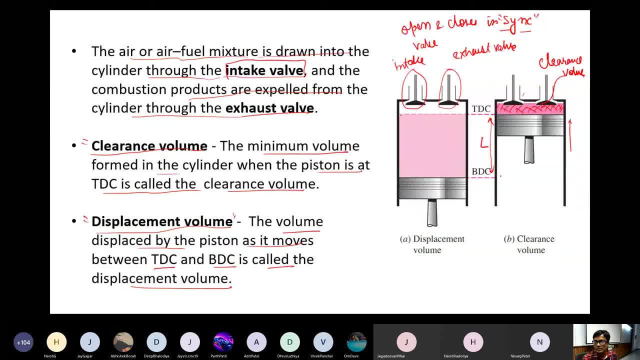 this area. So this is your diameter, bore diameter. So L times pi d by 2, whole square whole. So this is your L pi L d square by 4, am I correct? So this is your displacement volume. 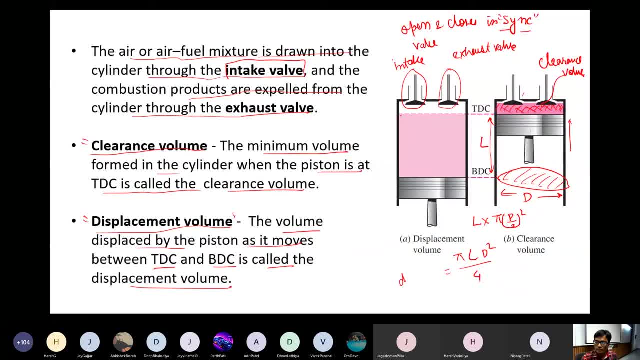 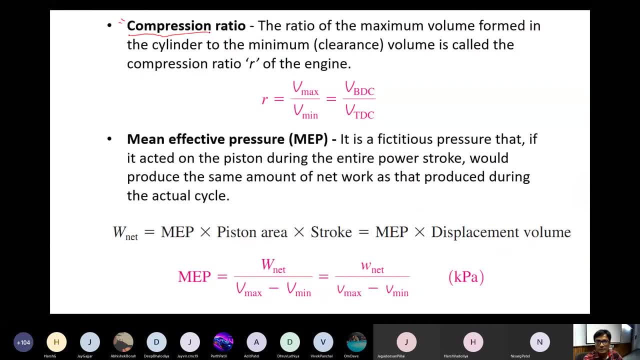 will see in the numerical example so that it will be more clear to you guys how to take up new methods. So these things we will often encounter we will see in the numerical example. uh, engine study is the compression ratio, the ratio of maximum volume formed in a cylinder. 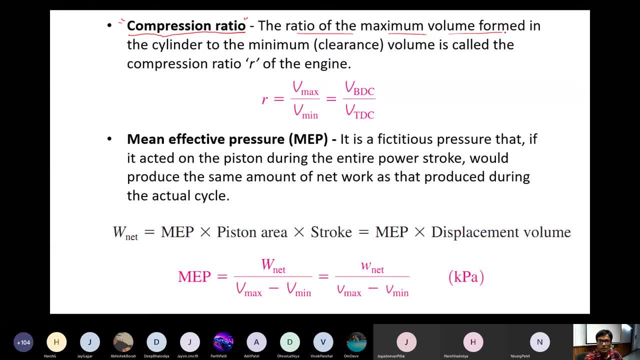 to the minimum clearance volume is called the compression ratio of the engine. so essentially this is the v max by v in v min. so v? v max is what volume at bottom dead center, the whole volume divided by at when tdc. so tdc is your clearance volume. so the whole volume from vdc to 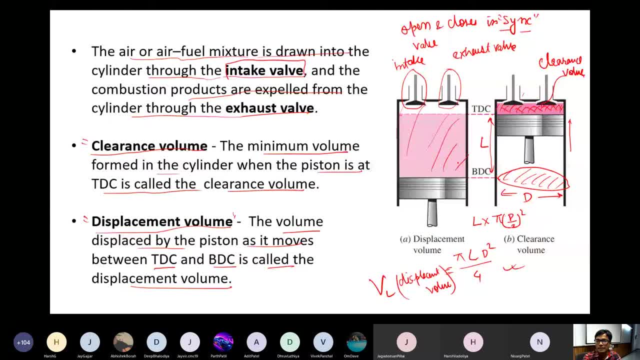 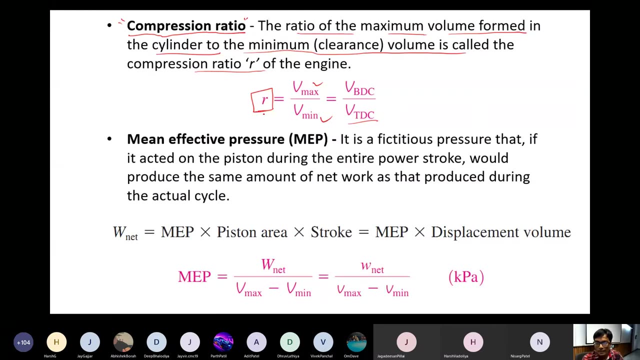 here divided by the clearance volume and volume at tdc is called the compression ratio of the engine. so we you should not be confused with the pressure ratio, which we will look into in the next lecture later later, later chapters, i mean later topics. okay, there is something called a mean effective pressure. so mean effective pressure is what this? 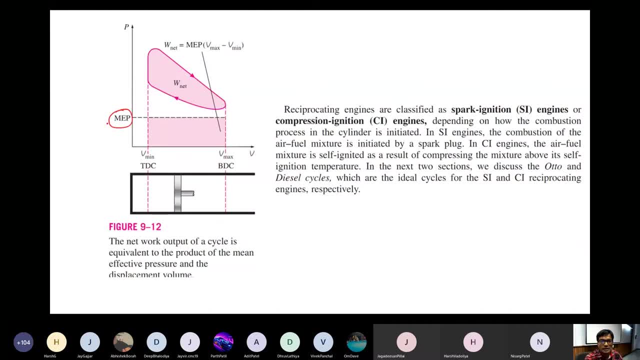 is a fictious. so this mean effective pressure. so let's suppose i'm i'm making some process in some some process in pv diagram, so this is my process that is happening. this is one cycle is happening, so to calculate the area so work or the work produced by this particular cycle so work is nothing but. 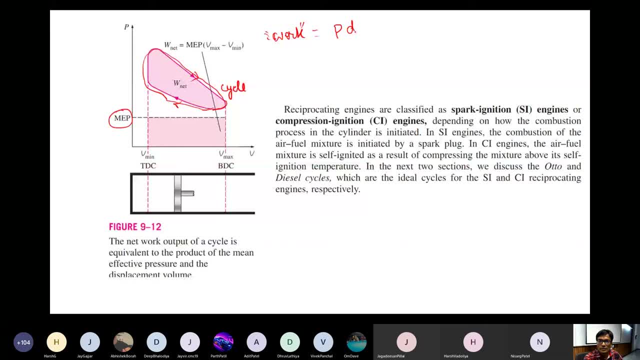 a pressure times, pdv, right. so this is what your, this is your, this is your real pressure. okay, but in in your engine, the pressure inside your engine may be fluctuating in nature, not maybe it's actually fluctuating with time. so p is a very, may be a very prominent function, function of time and space as well. 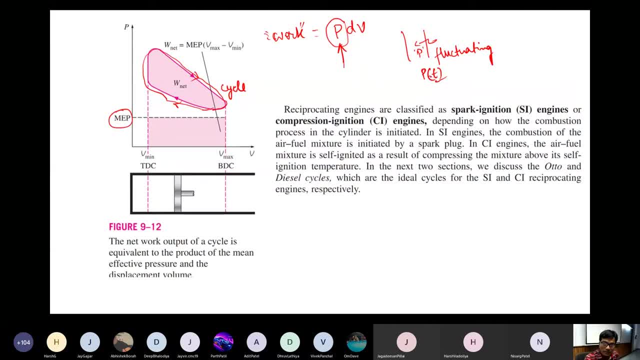 okay, x and t. so it it usually we. you cannot, i mean, calculate work efficiently if you take this p as a function of x and time. so what we do instead we take up a fictious pressure, so this is called mean effective pressure, and what it does just by multiplying this p. 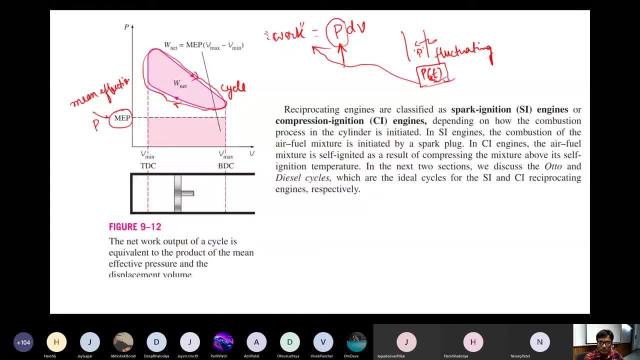 p times this change in volume, you will get the same work. this is equal to the same work, what you would get by actual cycle, right? So in a way, we are hypothesizing one pressure in such a way that you will get the same work out of it. ok, So it is defined as it is: a. 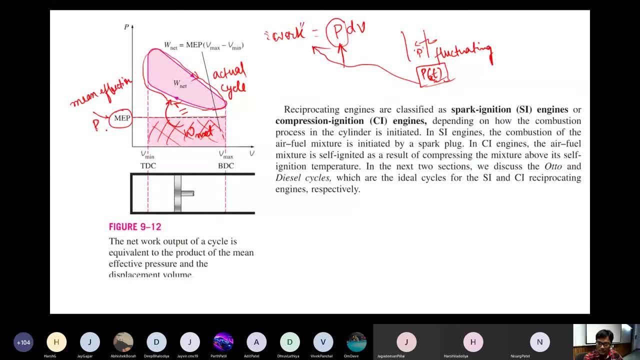 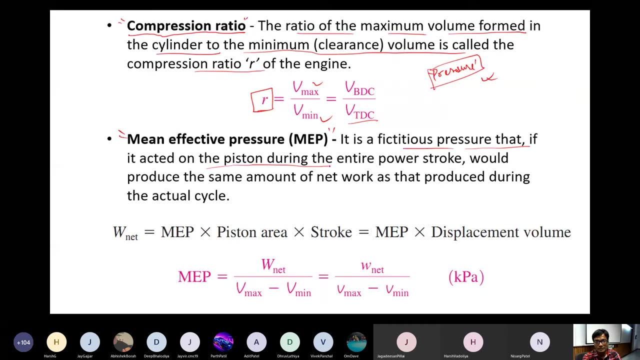 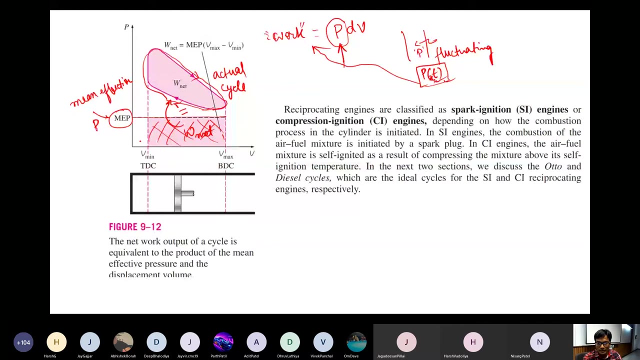 fictitious pressure, if it is acting, acted upon the piston during the entire power stroke, would produce the same amount of net work as produced during the actual cycle. ok, If you multiply this P dv you will get the work and actually also you will be getting the same work and so work net. So here I can do the math: work net is equal to P, or 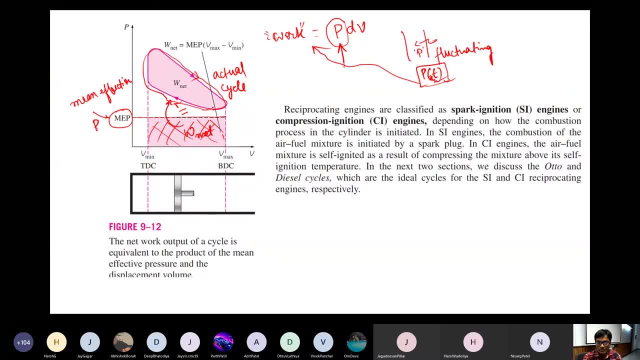 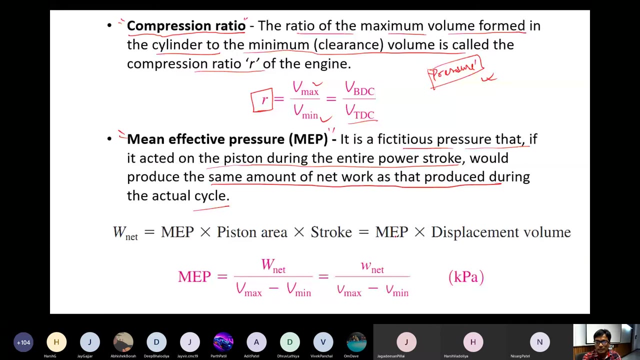 MEP, to be more precise, mean effective pressure times, The change in volume. So what is your change in volume? Piston area times the stroke or the displacement volume or whatever the volume you have, displacement volume. So V, L, this is displacement volume. we have already seen that this is your displacement volume. what 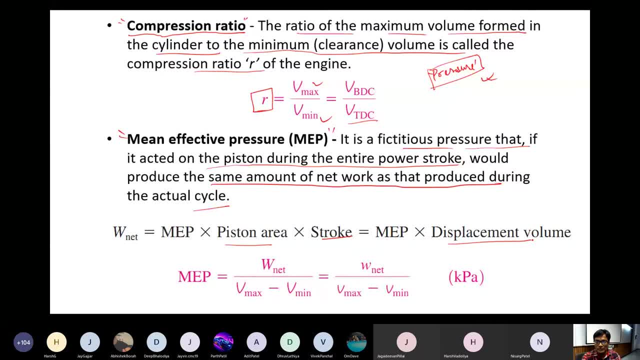 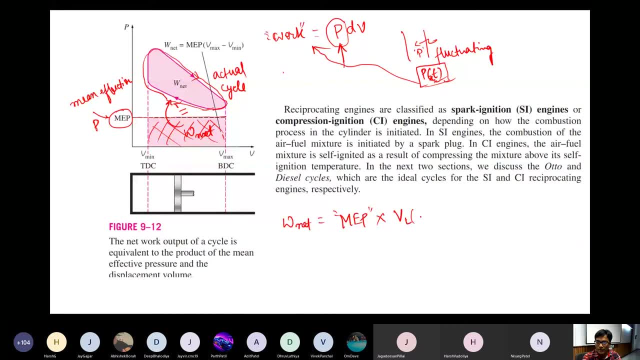 we talked, yes, this one. So if you multiply with P, you will get W net. So MEP can be defined as W net divided by displacement volume. ok, So this is your formula for that. So, but let us keep in mind that this is a 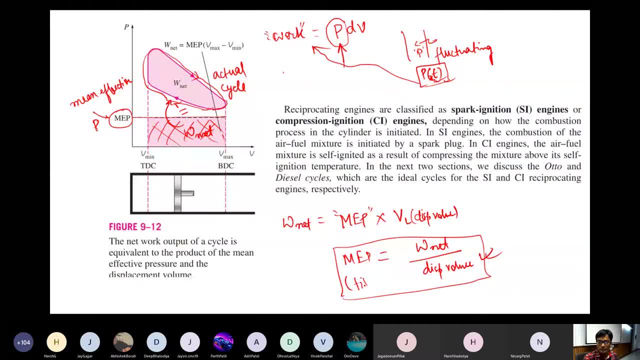 fictitious pressure, So it does not actually work, but we somehow we approximate it through the linear function So that we can calculate it easily. ok, So these reciprocating engines are classified as spark ignition engines and compression ignition engines, depending upon. 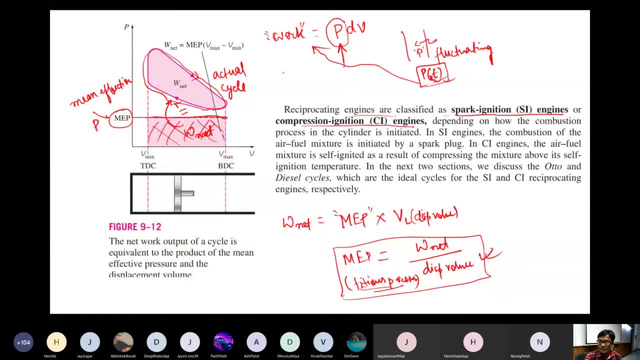 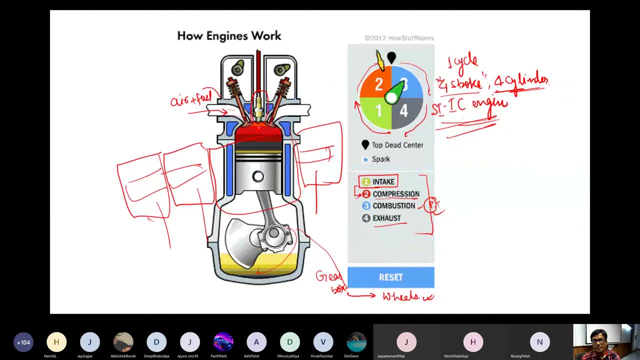 how the combustion process in the cylinder is initiated: The SI engines, the combustion of the air fuel mixture initiated by the spark plug, what we have seen over in this particular animation. So the spark plug is here and I have not shown the diesel engine over here, because in the diesel engine. we do not need a spark plug where air fuel mixture is self ignited, as the mixture above it is the self ignition temperature. So the pressure is brought so high so that the air fuel itself self ignites without having spark plug and those kinds. 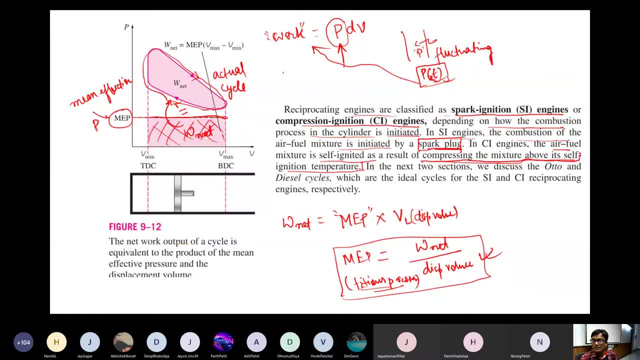 of engines are called compression ignition engines. In next two section we will discuss auto and diesel cycles based on your. I mean SI engines are typically based on the ideal auto cycles we will look into and these compression ignition engines are based on diesel cycles. ok, And we will look into in more details. 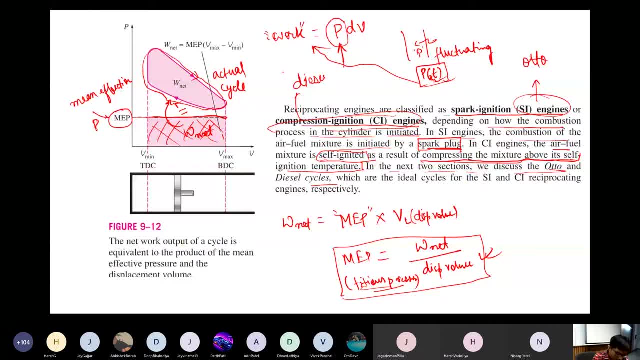 Ok, so then we will finish this also. The next thing we are going to talk about is the air standard assumptions, So there are few assumptions that we need to make up first in order to actually work with these auto diesel and all those sort of cycles, unless 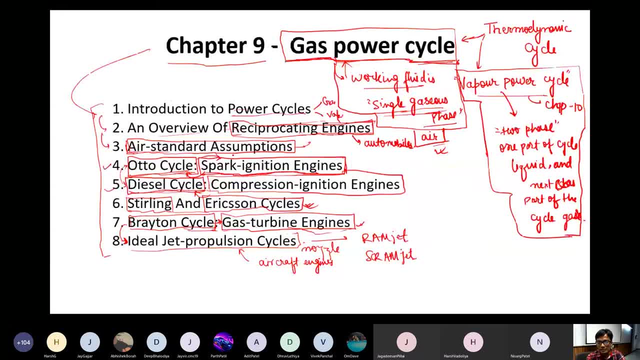 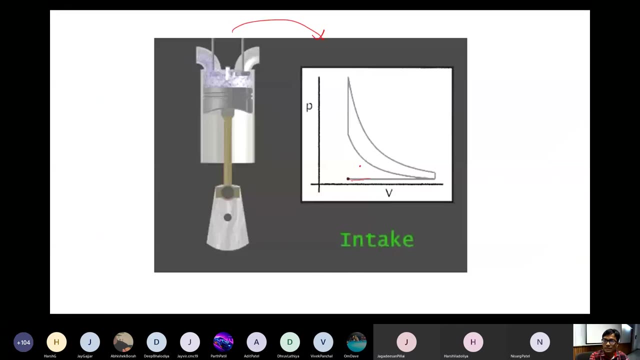 and until we are going to assume air in certain specific manner, we are not going to apply our analysis. ok, Ok, What are those assumptions? So you can see in, actually air and fuel are being burnt into the combustion chamber in your piston cylinder volume and combustion products are being coming. 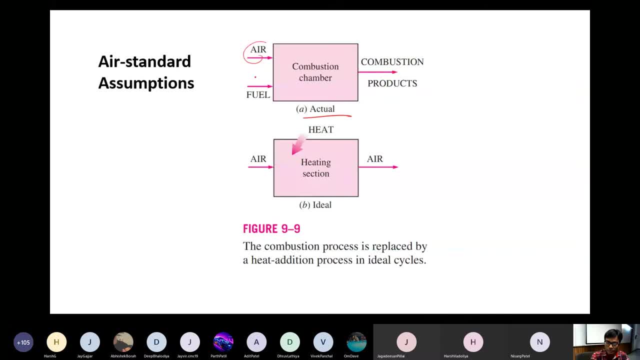 out. But in ideal case, what we will do, what we will assume, is that air is being heated by in some sort of heating section and the heated air is being coming out. So the combustion process- Ok- Is replaced by the heat addition process in ideal cycles. But the combustion process 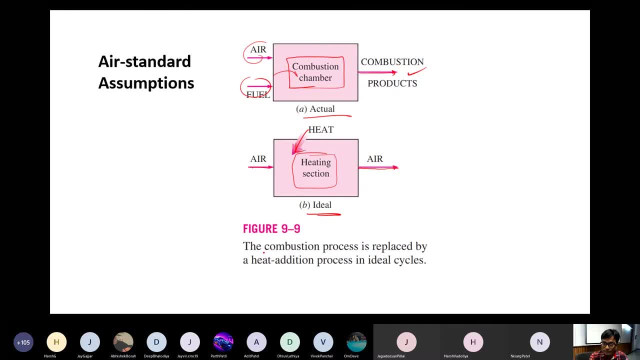 may have very complex phenomena and we are not going to look into those complex behavior of burning of O2 with some fuels, ok. And we are not going to look into- I mean into the micro, Ok, But for molecule wise, what is happening inside, We are not going to do, seek anything chemically. 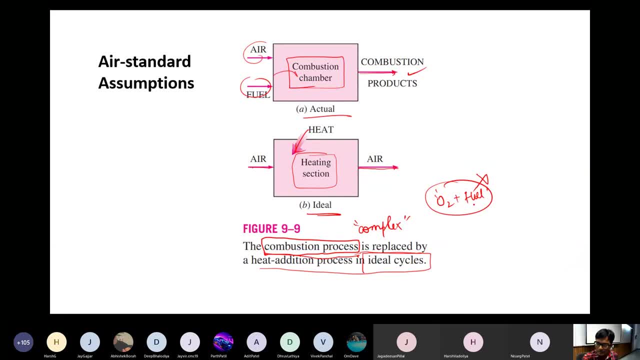 here Chemical analysis. no for us, for in this particular course, we are not going to do the chemical analysis. what is happening and why I mean those things are happening chemically? we just will replace this combustion thing, Ok, Ok, with actual, I mean this heating of the air, in order to do the analysis for ideal cycles. 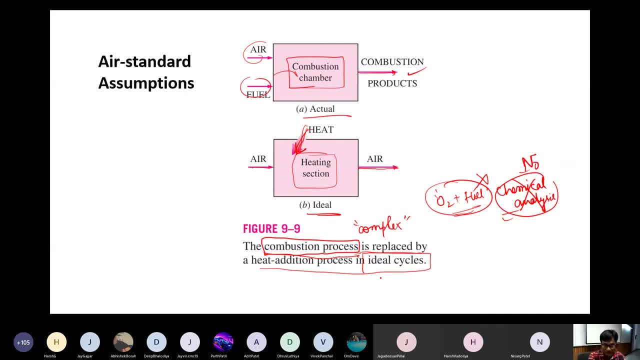 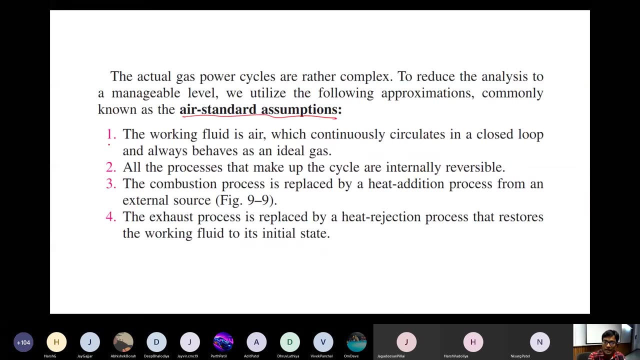 So there are a few assumptions that we are going to make and which are, namely, which are? there are four assumptions. The working fluid is air, which continuously circulates in closed loop and always behaves as an ideal cycle. this would be my first assumption, So my ideal gas loss. 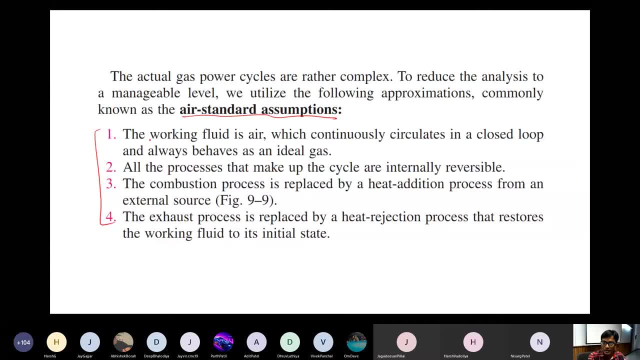 gas equations. we can actually make use of our ideal gas equations. here we are going to tell that my air is being treated as ideal gas and this makes no error in that, because the pressure and volume Inside the internal combustion engine is in the range- in the sufficient range so that we can 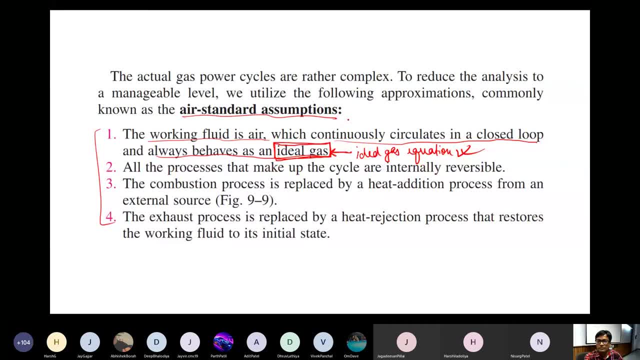 actually safely assume that air can be ideal gas. All the processes that make up the cycle are internal reversible. the processes are internal reversible in nature. there is quasi-static, slow and steady process is happening internally. The combustion process is replaced by heat addition process. 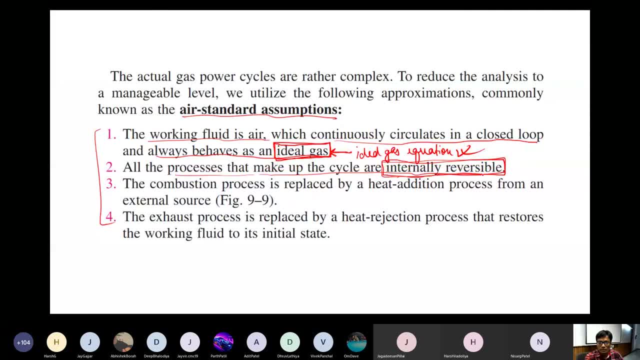 So from an external source. so this we have already seen. The exhaust process is replaced by the heat rejection process. So this is one heat addition process that is happening: combustion process and exhaust process is the heat rejection process that restores the working fluid to its initial states. 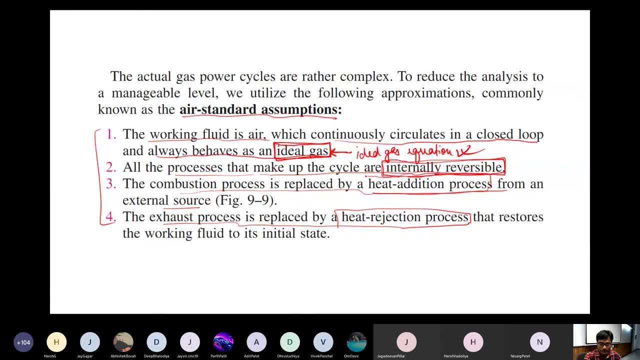 So this is very big thing. So actually, your cycle is going from one inlet or it is going something like this and it is coming again to this. ok, just going this and coming again to this. but in doing so we assume that by rejecting the heat last, at the last stage, it restores the working. 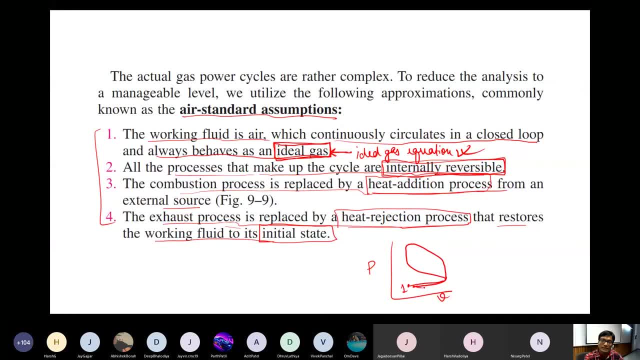 fluid as initial state. So we are going coming at the same place here. So then we you can actually think of your process in. ideally, you can actually replace this actual cycle with the idle cycle, some idle cycle. So these cycles will be may be autocycle or diesel.